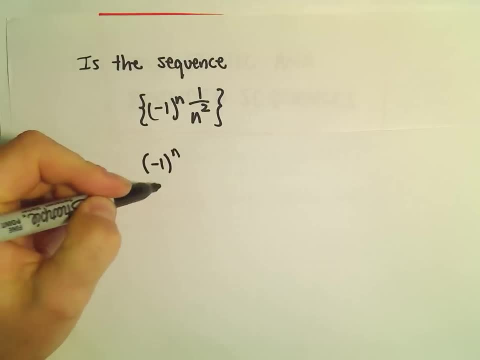 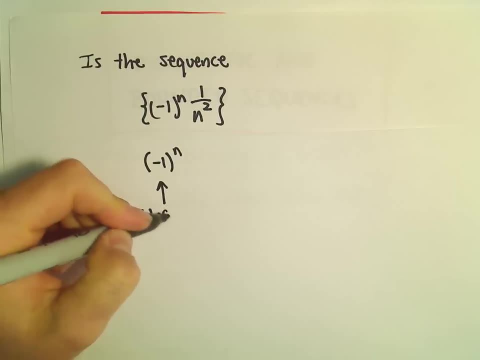 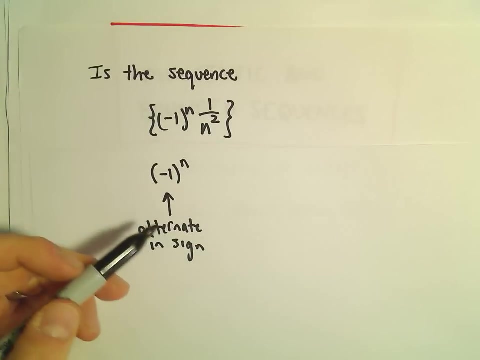 I mean, you know this negative 1 to the n, basically, as n increases, all that's going to do? it's going to make the sequence just alternate in sign Well. that to me makes me automatically feel like it can't be strictly increasing or decreasing. 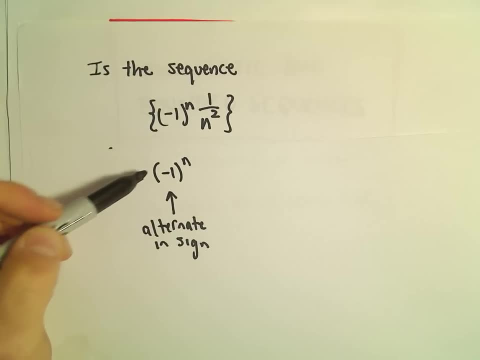 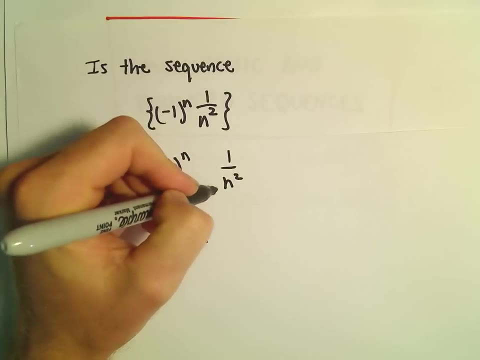 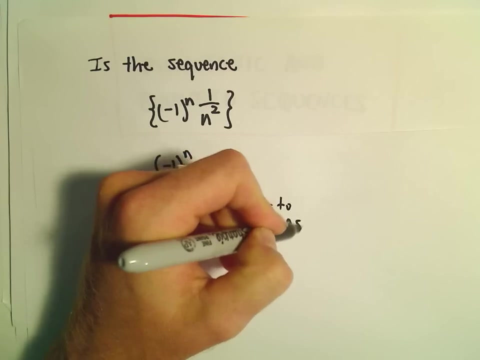 because it looks like it's going to bounce back and forth between you know, negative, positive, negative, positive. So it's not strictly getting bigger or smaller The 1 over n squared, if you think about that. this just gets closer to 0 as n increases. 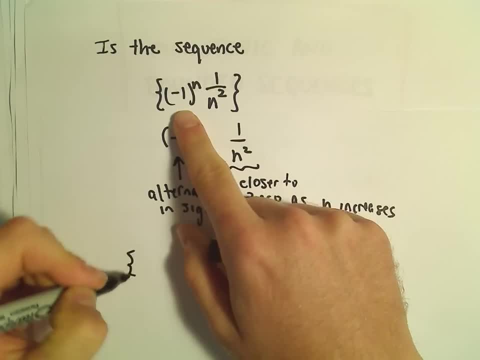 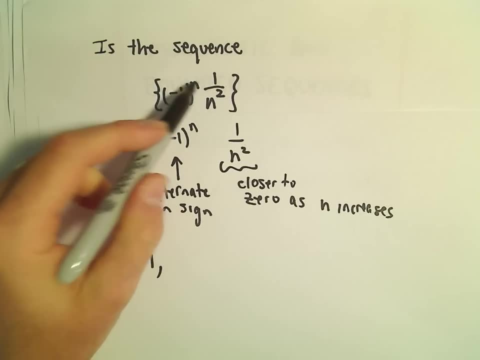 You know so and you can even plug in numbers. If we plug in 1, you know we would get negative 1 times 1 over 1.. So we would get negative 1.. If we plug in 2, we would get a positive 1 over 2 squared, or a fourth. 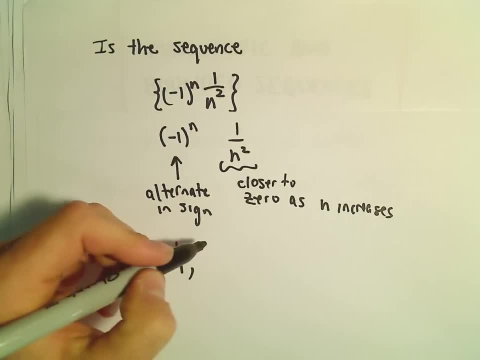 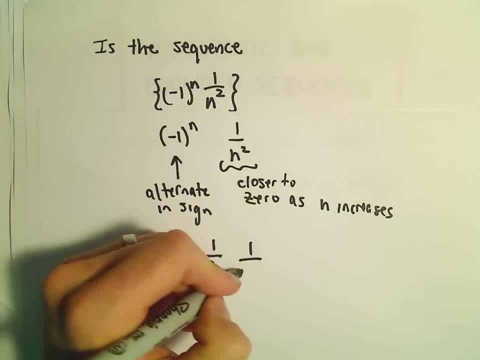 If we plug in 3, we would get a negative 1 over 3 squared, which would give us negative, Negative 1 over 9.. And then positive again. if you plug in 4, we'll get 16,, et cetera. 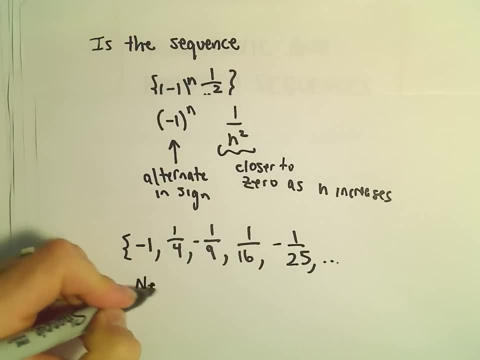 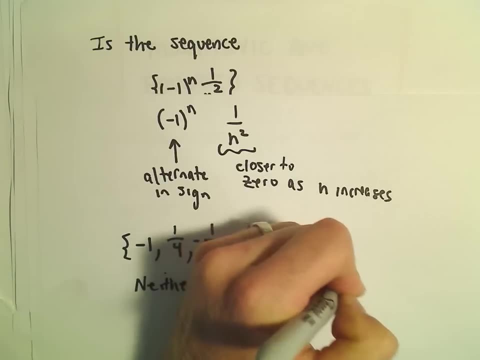 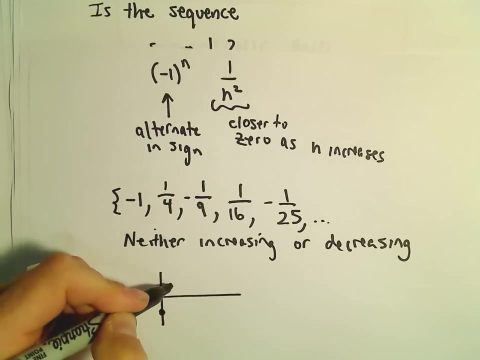 So it's, you know, it's clear to see that this is neither increasing or decreasing, You know, and again you're starting like at negative 1, and then you're up at a fourth, a negative 9th, a 16th. 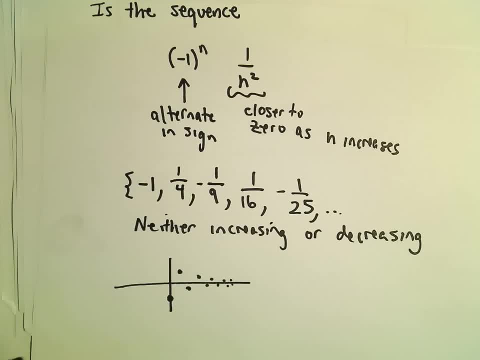 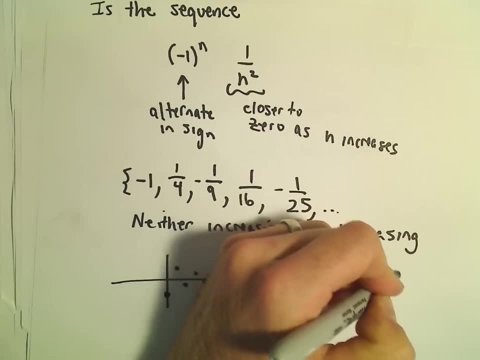 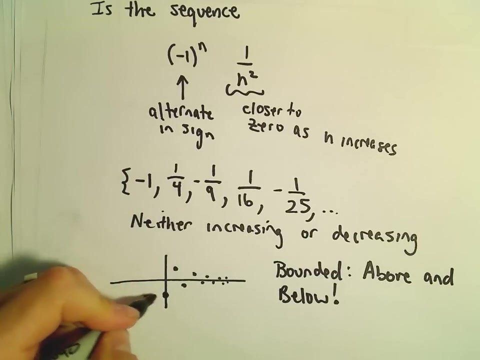 But if you think about it, okay, so it certainly looks like to me it is bounded. It's going to be bounded to me both above and below, And to me it looks like it's going to be bounded below. You could say it's bounded below by negative 1.. 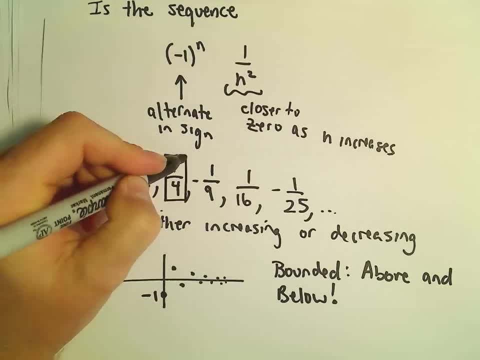 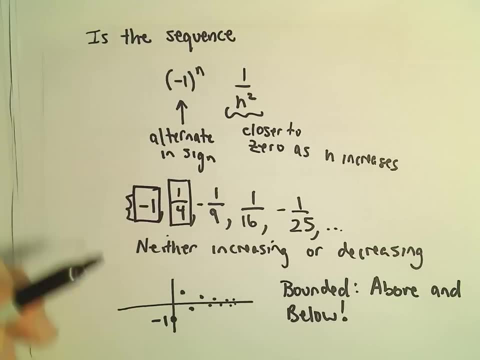 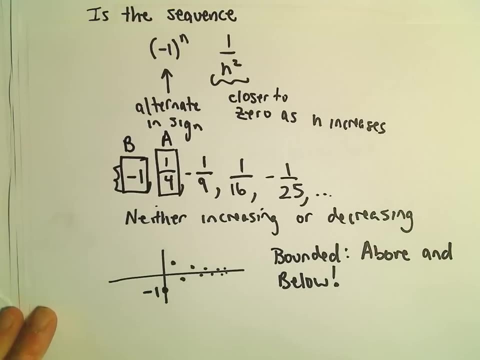 And then it's bounded above. It looks like the biggest positive number you would ever get out of our sequence would be positive 1 fourth. So it's bounded below and above by both of these numbers. Again, if a sequence is neither strictly increasing or decreasing, 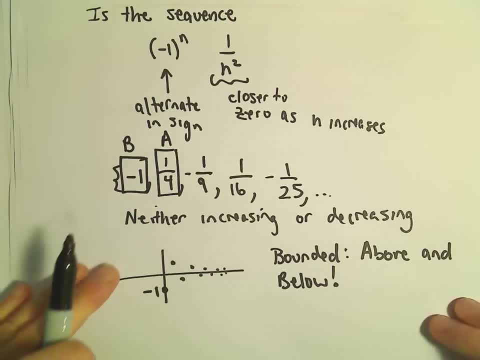 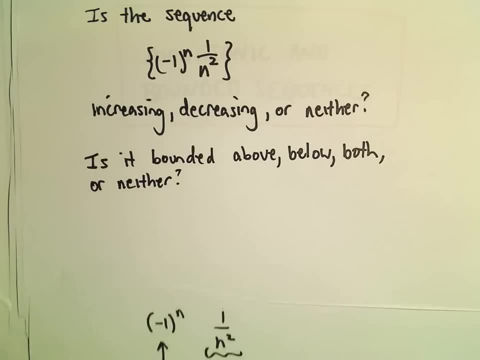 and is bounded above and below, you know. in that case you can't really say for sure that it converges or not. The question isn't asked: does the sequence converge? but we could always address it. I think it's pretty easy to see that it's going to converge to 0..